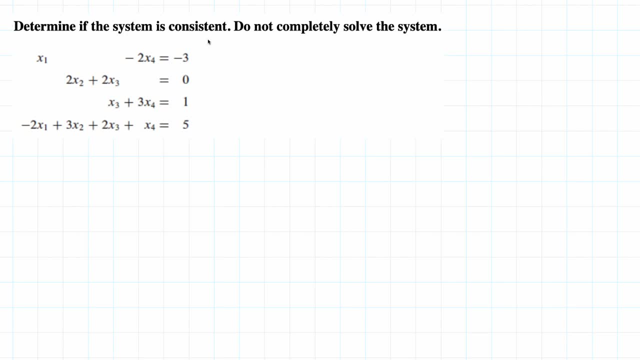 Determine, determine if the system is consistent. that means if there is at least one solution. okay, we know that when we have a system of equations, linear equations, we can have no solution. that is inconsistent system, or we can have one solution or infinitely many solutions that is consistent. So here we need to check if this system is consistent. 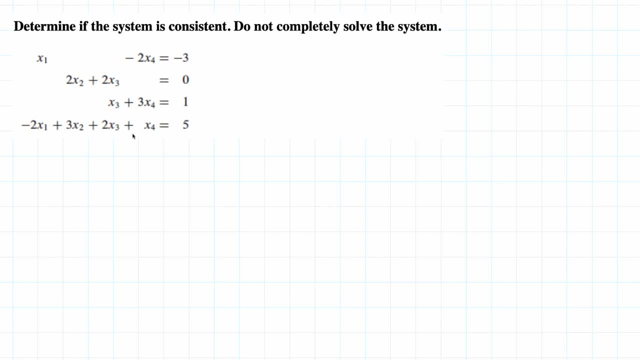 Do not completely solve the system. that means we don't have to find the exact values of x1, x2, x3, x4. there are four variables, So first we're gonna write down the augmented matrix, okay, so the matrix of coefficients. and the last, these are constants, So one. so x1, x2, x3. so first, 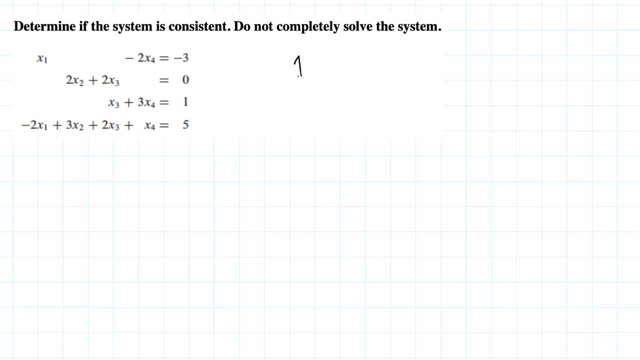 look at here: first equation: There is one, no x2, no x3, so we can put zero. zero for x4 is negative two and finally negative three. okay, now we can put colon here, not needed. for the second equation: there is no x1, so zero. 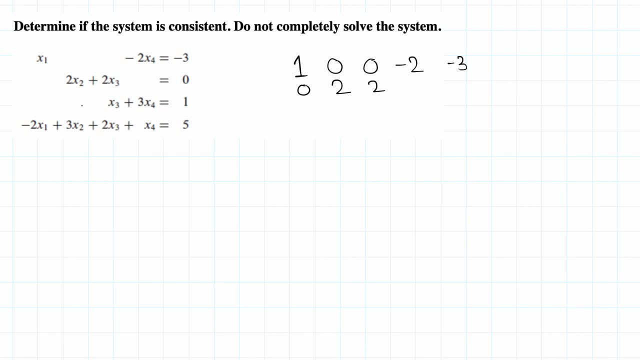 two, two. there is no x4. oh, it's kind of given nicely. so zero, zero. third equation: plus two variables are absent. so one, three, one here negative two, three, two, one and five. okay, this is the augmented matrix of this system. Now our goal is to make there is some type of 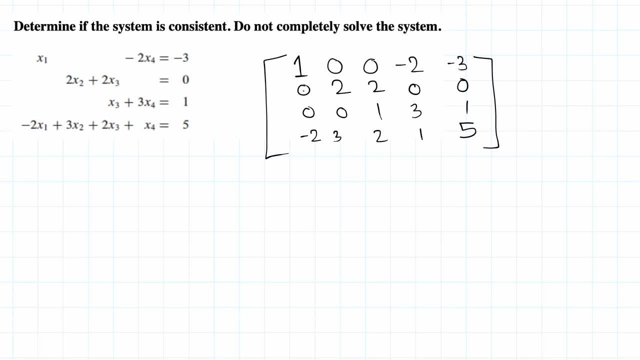 number and here zero and something- okay, this is good. And zero, zero one- oh, this is also good. so we want to make this triangular matrix, so we want to make zero, zero, zero and we can have any number here. First three rows are good. okay, it's already. 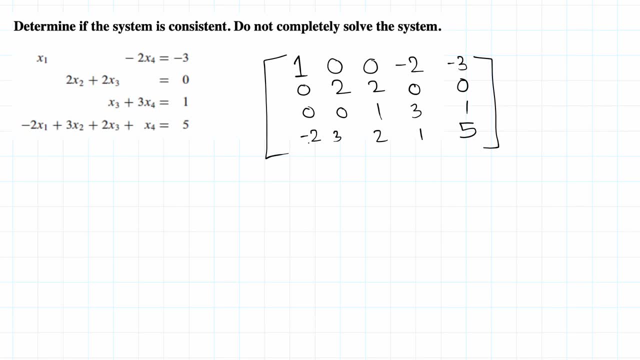 triangular, but we need to make this zero using elementary row operations, and then this zero, then this zero, so and we can have some number here. okay, So we're going to work on R4. let me write on R4. so that means R4 plus to make this 0, we multiply R1, because that's the easy one. 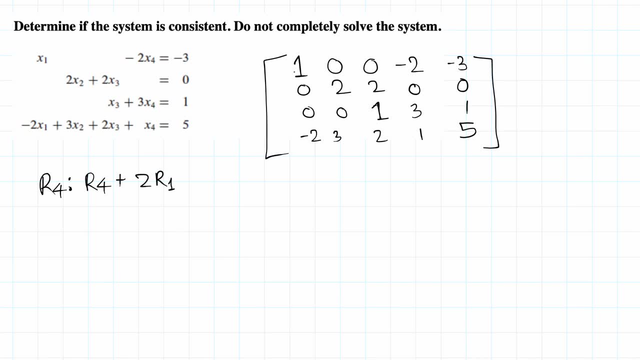 H1 multiplied by two R1, so this will be 2 plus negative, 2. negative 2 plus 2 will be zero. okay, so we do one at a time. that makes so we are only changing R4. so first three rows are same: 1 0, 0. 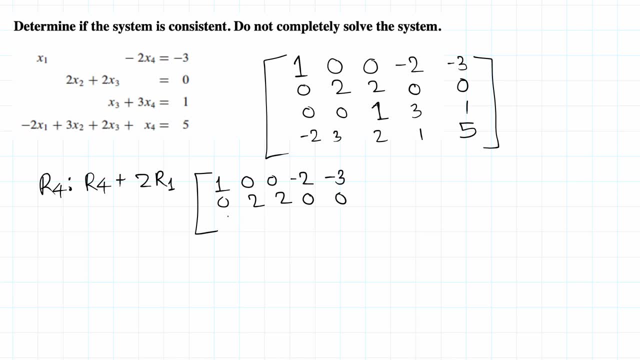 0, 2, 2, 0. 0. 0, 0, 1, 3, 1.. Now here. okay, we need to do this work. negative 2 plus 2 times 1, 2, that is 0, 3 plus 2 times 0, which is 0, 3 plus 0, is 3, 2 plus 2 times. 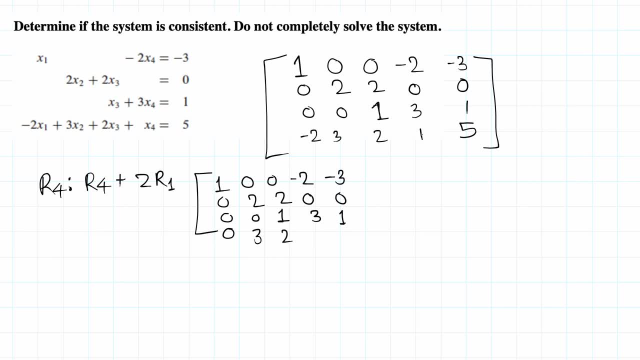 0 is 0, so that's 2, 1 plus 1 plus 2 times negative, 2, negative: 4, 1 plus negative. 4 is negative 3, okay, and 5 plus 2 times negative 3 is negative 6, 5 plus. 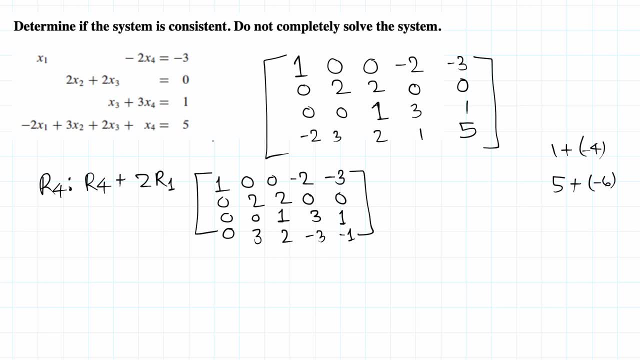 negative 6 is negative 1. okay, So we are able to make at least this one 0, the first zero. Next, we need to make this 0, so we are still working on r4. it's the row 4, that's that's where we have issue. okay, and that is r4 plus. okay, we can take. 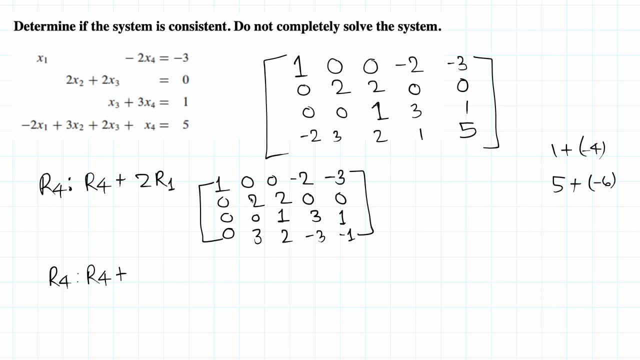 help of second row, because there is a term here there's 0, so, no, no help. so, okay, it's not that easy because 2 and 3. so to make this 0, okay, we can multiply this by 2 times. let's say, if I multiply by 3 halves, then this will be 3 and 3. 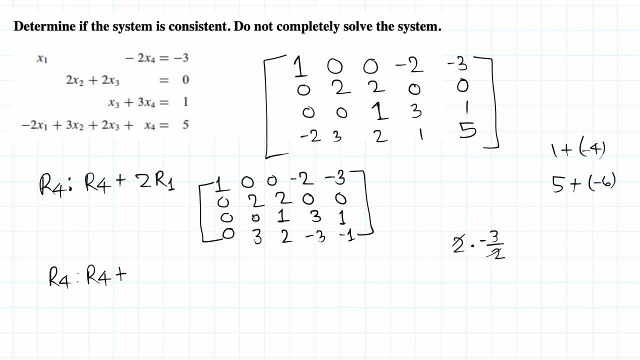 okay, how about multiplying by negative 3 halves? okay, so we need to experiment: 3 plus. if we multiply this by negative 3 halves, then we get negative 3 and 3 plus negative 3 will be 0.. So r4 plus. multiply r2 by negative 3 halves, because 3 plus. 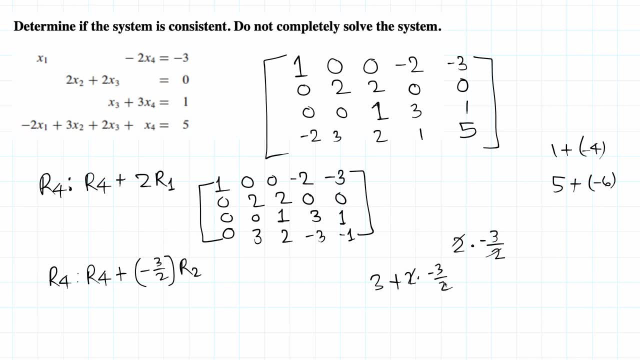 2 times negative. 3 halves means 2 to cancel. 3 plus negative 3 means 0. okay, that's how we get 0.. So or we could have multiplied second row by 1 half. multiply by 1 half, that would have 0.. 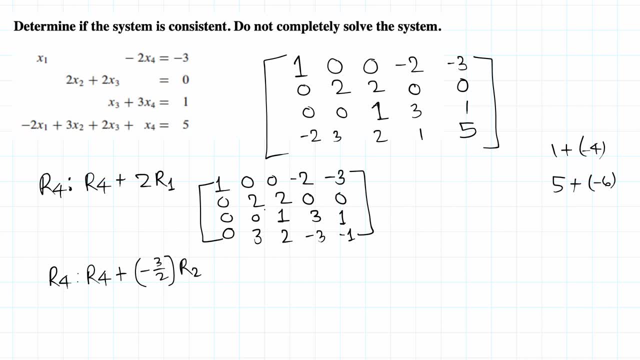 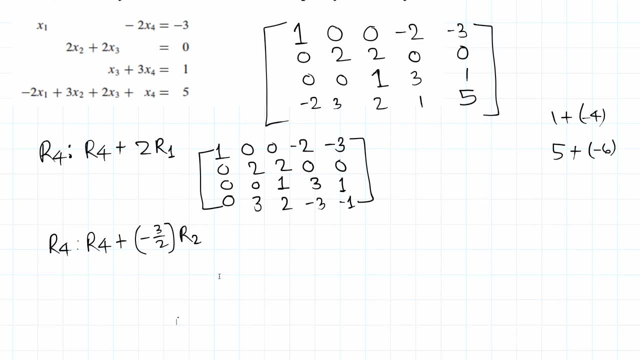 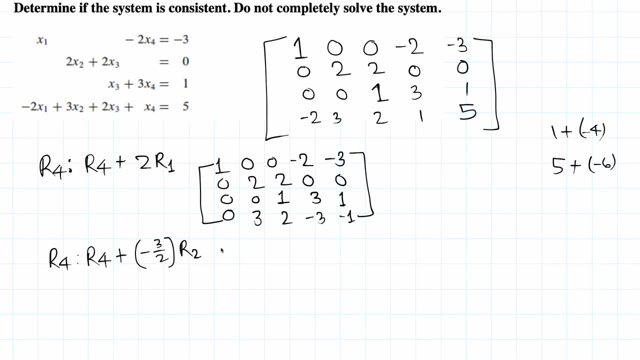 then 0, 1, 1, 0, 0. okay, that then it would be 1. then we could have multiplied by negative 3, ok, so there is an option, but let's do this one, ok. so here now we are leaving. first three rows is 0, 2, 2, 0, 0, 0, 0, 1, 3, 1 here. 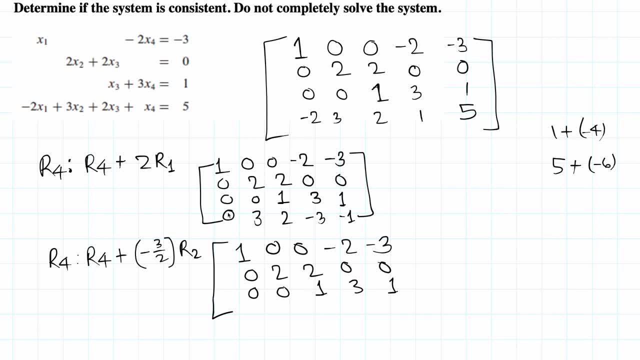 0 times any number. I mean 0 plus. we are multiplying here, right, r2. okay, here is 0, so 0. this is 0, 3 plus 3 plus here negative 3 halves times 2. okay, that's 0. that was our design. now 2 plus 2 plus negative 3 halves times 2, 2 to cancel. 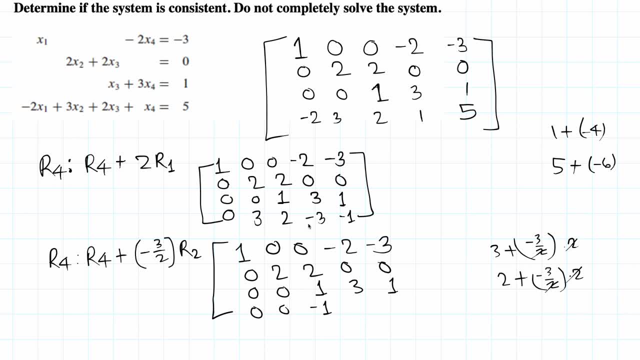 2 plus negative 3 is negative 1, now negative 3 plus negative 3, plus we multiply negative 3 halves times 0, just 0. and negative 3 plus 0 is just negative 3, now negative 1 times, again 0, changes does not change. so negative 1, okay, we. 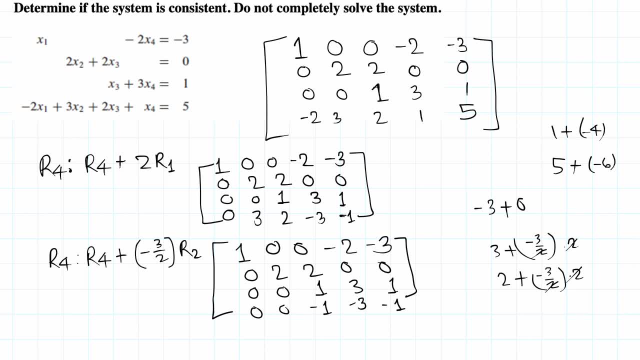 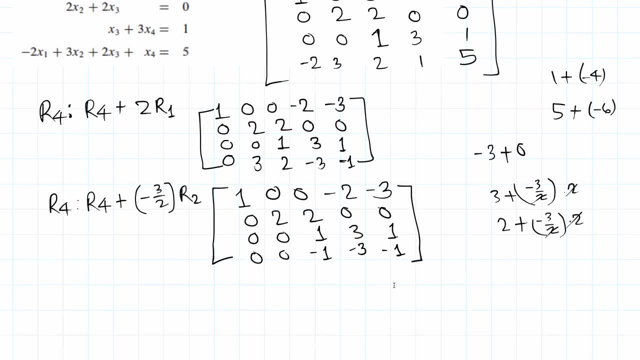 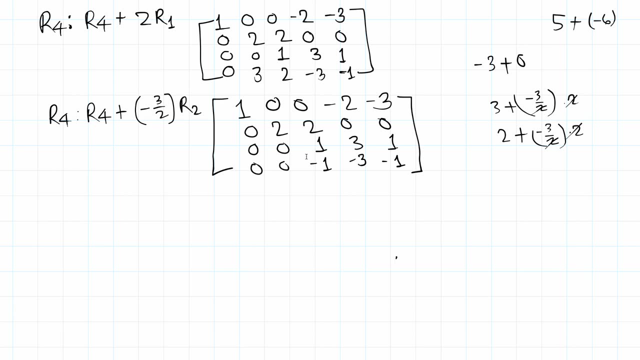 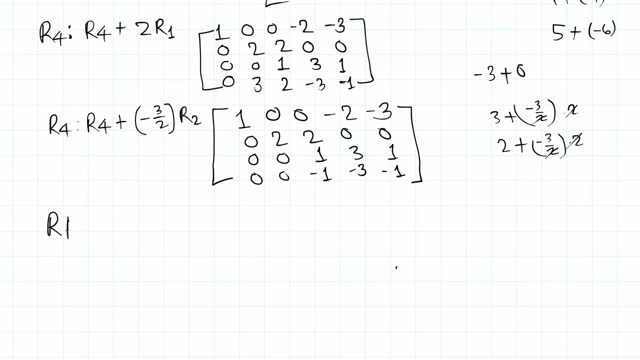 are almost there. okay, we have to make this augmented matrix triangle. And here is now we are here. okay, 0, 0, we have to make this 0 and we are all good, then this will be triangular. okay, still working on r4, we have to make this 0. 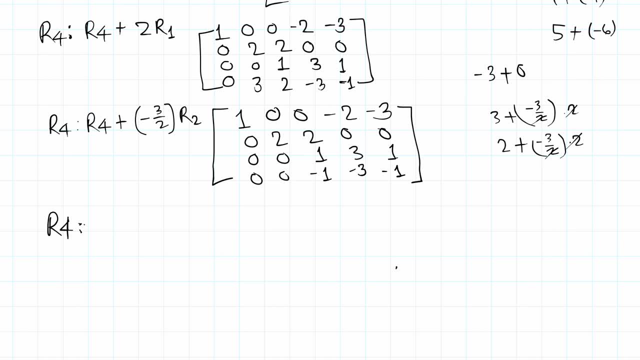 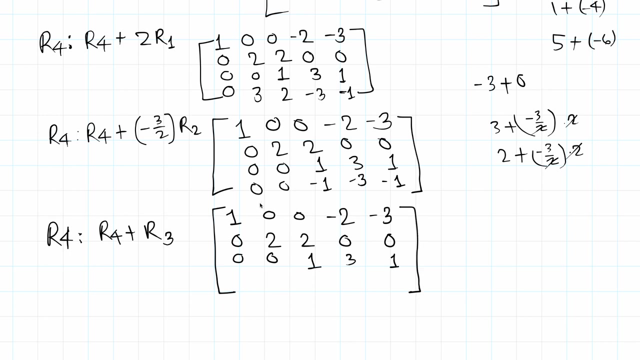 oh, here is 1 right, because 0, 0, 1, so r4 plus simply add r3. okay, First three rows are same, not changing R3, 0, 0, 1, 3, 1, okay. Now R4 plus R3. okay, we are adding R4 with R3, 0 plus 0, 0, 0 plus 0, 0, negative. 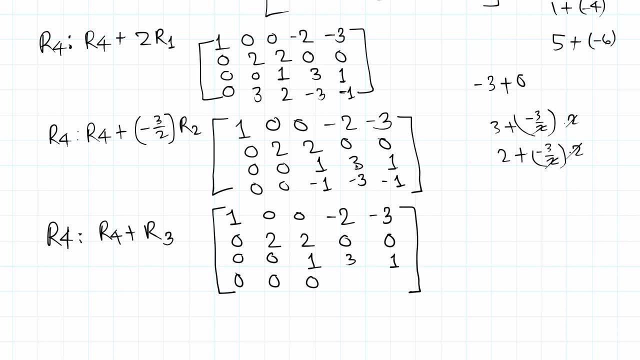 1 plus 1: 0, negative. 3 plus 1, oh, negative. 3 times negative: 3 plus 3, sorry, 0. negative 1 plus 0, oh, all 0.. Now to see if this has a solution. we can convert this. 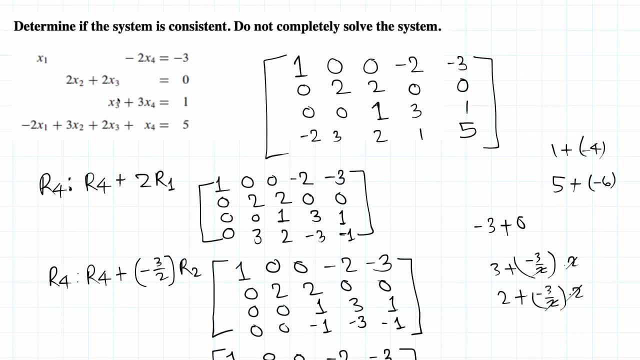 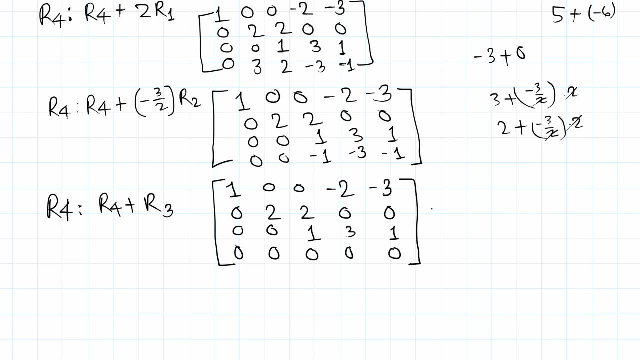 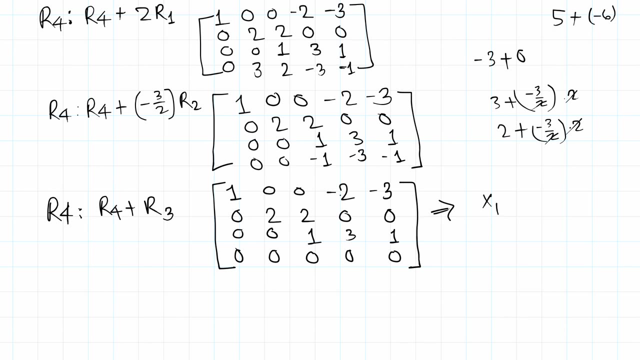 back to putting in terms of variables. let's make equations, okay. So this one was from. this one is, in fact, okay. pretty much. 1x1, x2, x3, x4 minus 2x4 equals negative 3, okay, we. 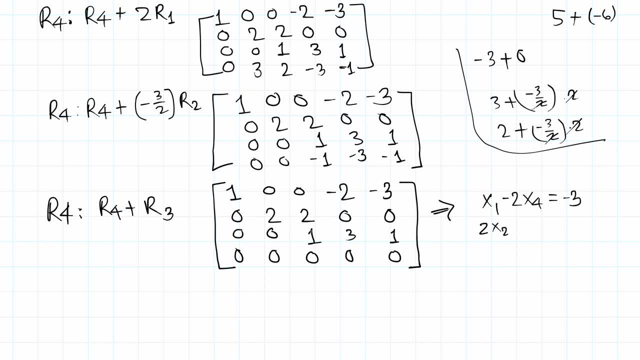 didn't change anything. and this one is 2x2, x3 plus 2x3, 0x4, so 0.. Third is x1, x2, x3 plus 3, 0.. x4 equals 1 and everything. 0, I mean there are nothing. And if we look at this, 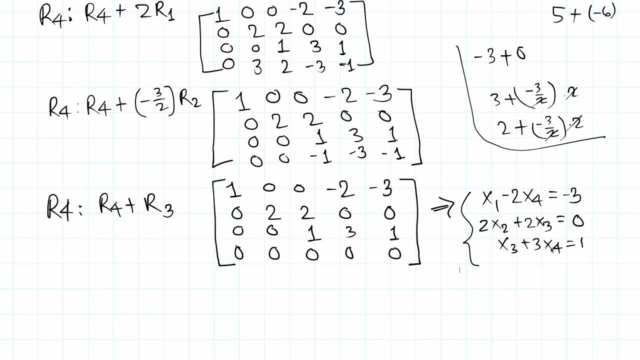 closely. so we got from here. if we look at closely, we can. from the third equation we can solve for x3, right, x3 would be 1 minus 3, x4, and when we can plug in x3 here, then we can solve for x2,. okay, that will be in terms of. 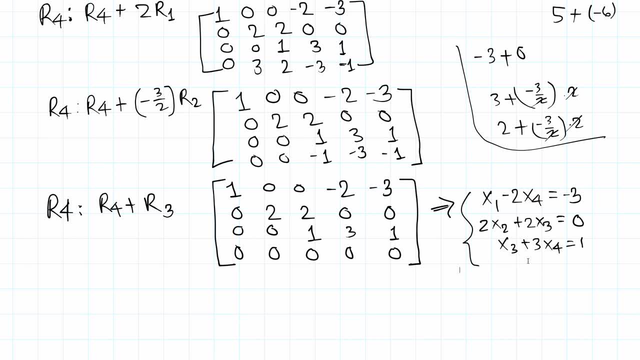 x4 and plug in here, then we can find x1.. By the way, there are four variables and we got three equations, so we learn in next section. in this case there will be infinitely many solutions, but this is good, so we have a solution that means.